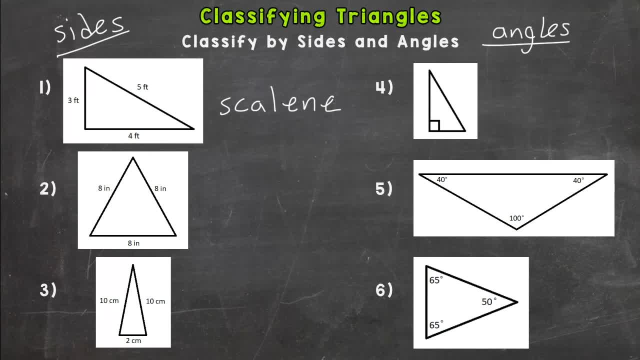 call that six Scalene. So this is a scalene triangle. None of the sides are the same. Let's go to number two. As you can see, all the sides are eight inches. All of them are the same. If they are all congruent, we call that type of triangle equilateral. 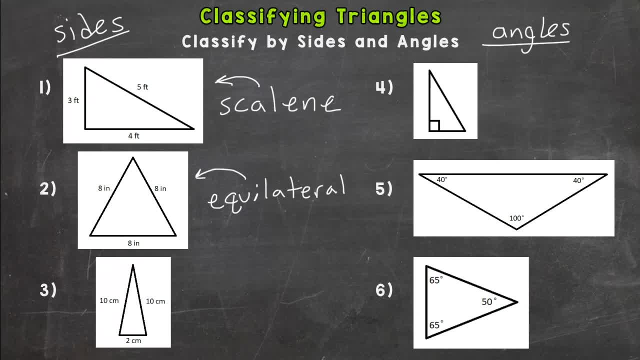 So this is an equilateral triangle. And then number three, your last option. here we have a ten centimeter, a 10 centimeter side and a 2 centimeter. So 2 of the sides are congruent. if two of the sides are congruent, Isosceles. So again, 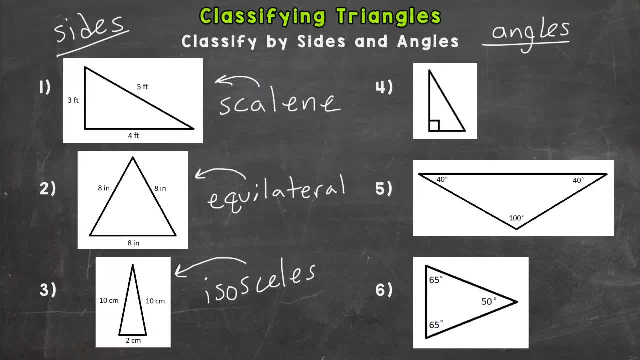 top one. number one, Scalene: none of the sides the same. Number two: all of the sides the same as equilateral. and then number three: two of the sides are Isosceles, All right. number four- Let's go with that to classifying by the angles. so, number four, on the bottom left hand angle you. 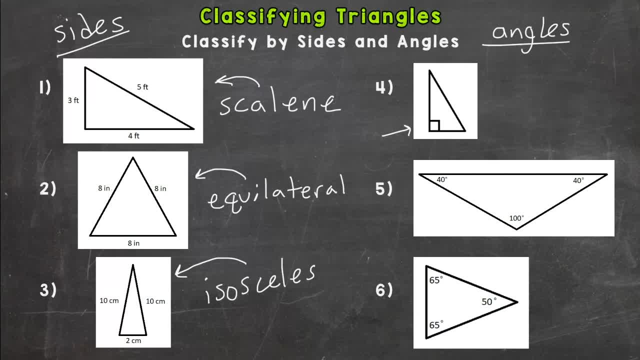 see a little box there. whenever you see that, that means you have a 90 degree angle in that triangle. if the triangle has a 90 degree angle, you call it a right triangle. a right triangle number five: we have angle measures of 40, 40 and. 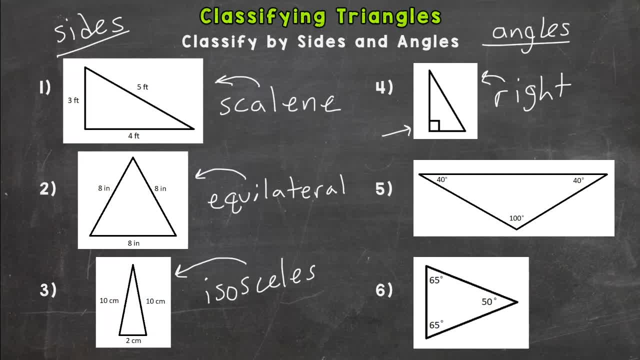 100. so do we have a right angle, a 90 degree angle, in that triangle? no, so it's not going to be a right triangle. so what we need to look at next is: do we have any angles that are over 90, or are they all under 90? well, we have one above 90. 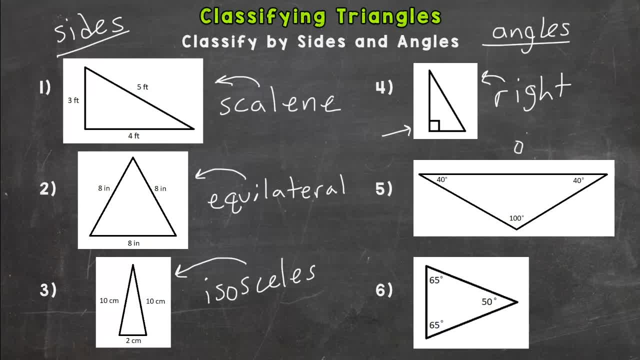 if you have one angle above 90 degrees, that triangle is called an obtuse triangle. and then the last one. let's take a look if we have any 90 degree angles, 65 degrees, 65 degrees, 50 degrees. so no, we do not have any 90 degree angles, do we?